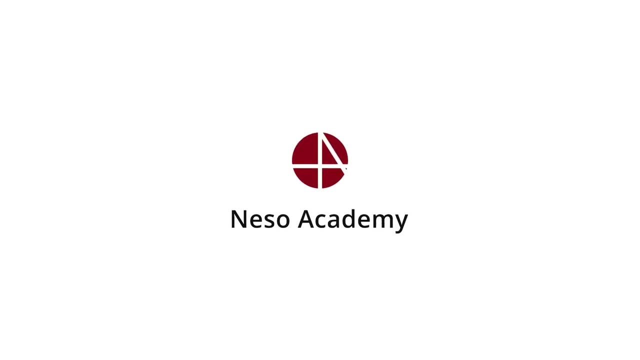 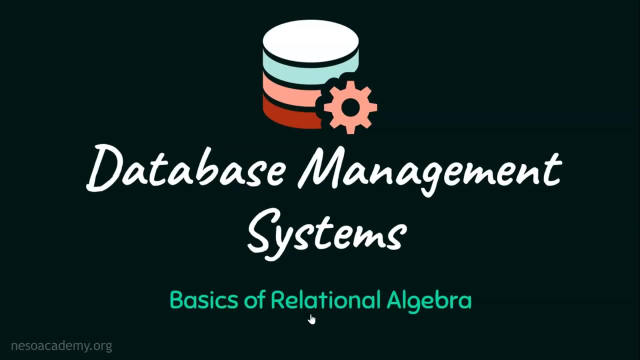 Hello everyone, welcome back. Algebra is one of the broad areas of mathematics. We would have come across various algebra branches. Let's take abstract algebra, where the abstract algebra is to study the algebraic structures such as groups, rings, fields, and abstract algebra has its wide 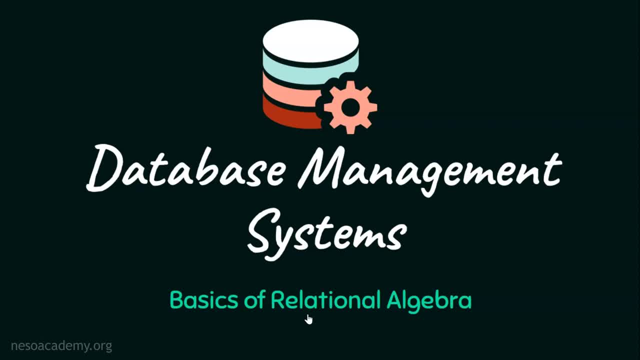 application area in the field of cryptography. Coming to linear algebra, linear algebra deals with the linear equations, linear mappings, and is used in the application area like the weather forecasting. Coming to Boolean algebra, these Boolean algebra deals with the variables that are, with the truth values- true or false- and Boolean algebra has its widespread applications. 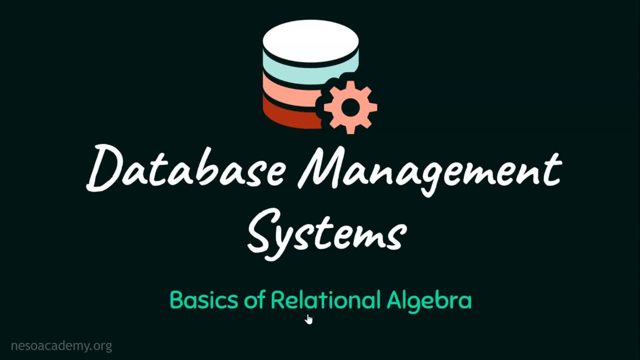 in the areas of digital circuitry designed in personal computers, pocket calculators, CD players, cell phones and other electronic products. One such algebra that we are going to focus in today's presentation is the relational algebra, and in today's presentation we are going 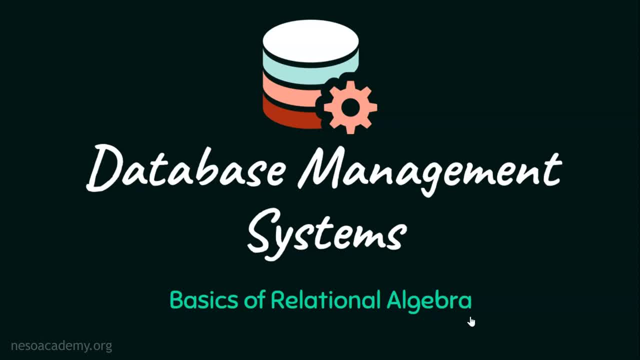 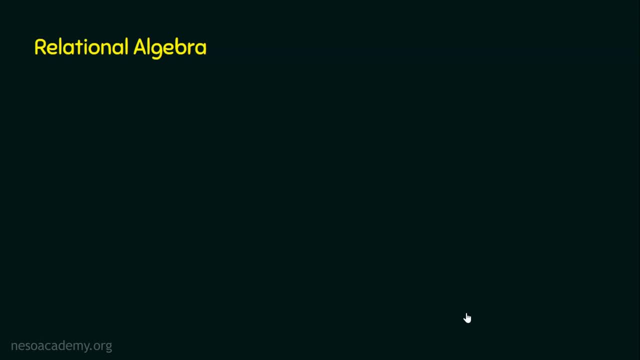 to focus on the basics of relational algebra. While waiting, let's step into the topic of the day: the relational algebra. And relational algebra is basically a procedural query language. What do we mean by this? It means we need to instruct what to do. 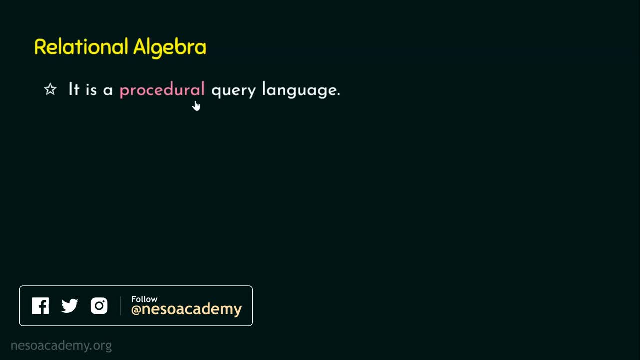 we are expecting the result from the database and the result is going to be a table or a relation. and in order to get that result- the table or the relation- we need to instruct what is required and how to retrieve that data or how to retrieve the result, and that is why we refer relational. 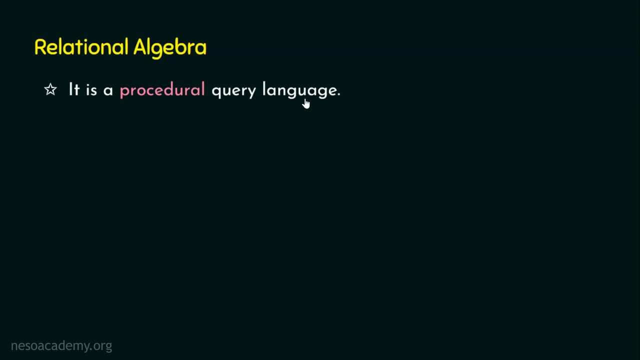 algebra as a procedural query language. If you are directly watching this lecture, I request you to navigate to chapter 1 of this playlist and find the lecture database languages, where I have explained about the database language If you are not familiar with the database language, 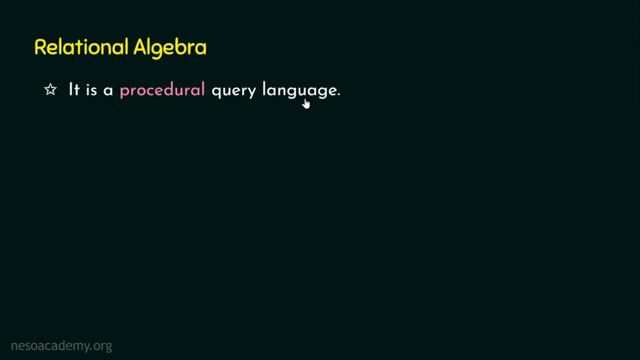 the database languages, the procedural query language and the non-procedural query language, with examples For now. just understand: relational algebra is a procedural query language and what it actually does. Basically a relational algebra is a set of operations on relations. This is like. 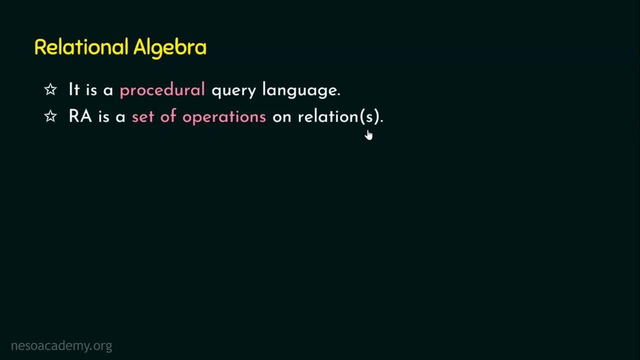 the normal algebraic operation where it's going to take input and it's going to produce the output. Likewise here also, relational algebra is basically a set of operations on relations, So it's going to work on the relation and does the operation and gives the result as a relation. 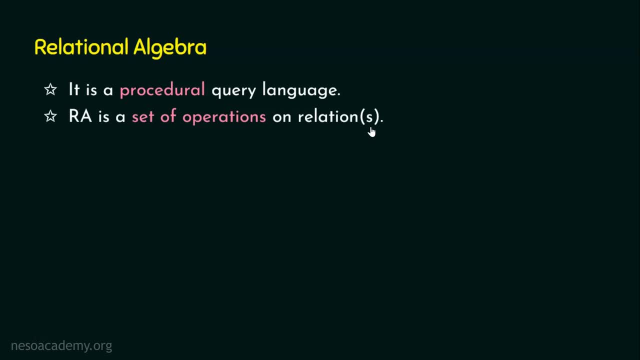 only, and that's why we say relational algebra is basically a set of operations and to be precise, it is like a set of algebraic operations. These algebraic operations, like the addition, subtraction, all these take some values as the input and does the operation and produces the 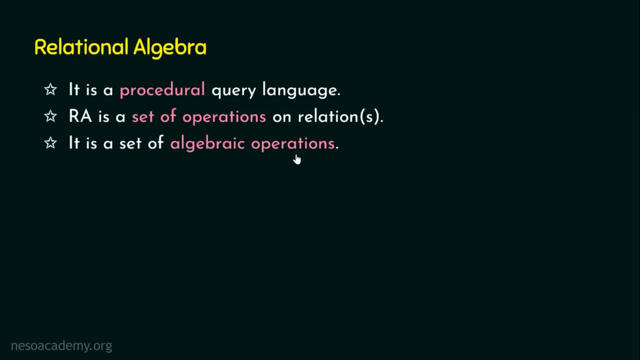 output. Likewise, here also, relational algebra is going to take relations, as input does the operation and generally it's going to take the output and produce the output. So it's going to take the output and do the operation and produce the output and generates the output which is also. 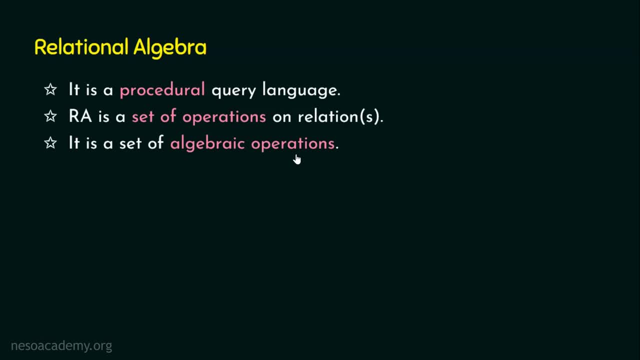 a relation. In simple terms, relational algebra is a set of operations which takes one or more relations as input and produces a relation as an output. So that's what the next point says: The input is going to be one or more relations and the output is going to be a relation. 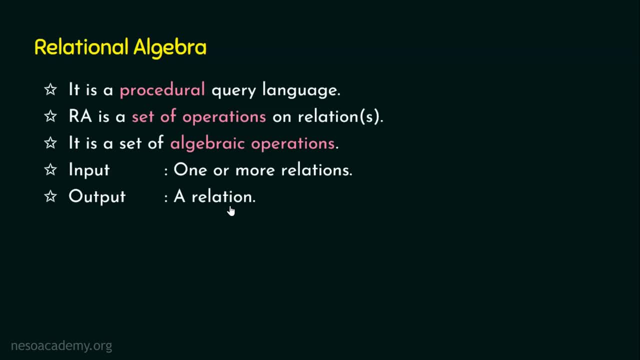 Why one or more relations? There are certain relational algebra operators which are unary operators, where it takes only one relation as an input. There are certain relational algebra operators which takes two or more inputs, So they are binary or ternary. So what I mean to say is: 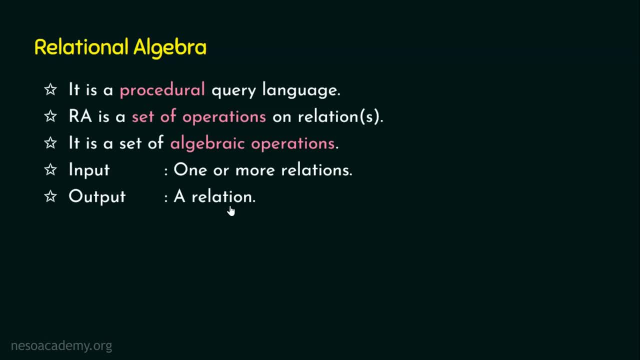 in a nutshell, it takes one or more relations as an input and produces another relation as an output. And why do we need to study this relational algebra? Because it provides a theoretical foundation for relational databases. We know the power of relational databases in this contemporary 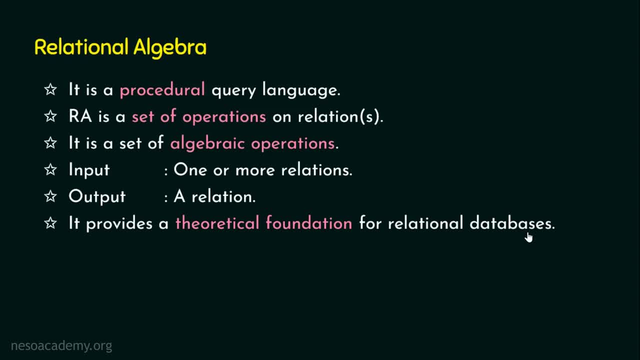 world When we want to work on the relational database or when we want to know the foundations of the relational database. it's always recommended to have a sound knowledge on relational algebra, because it provides a theoretical foundation for the relational databases, The well-known DBMS. 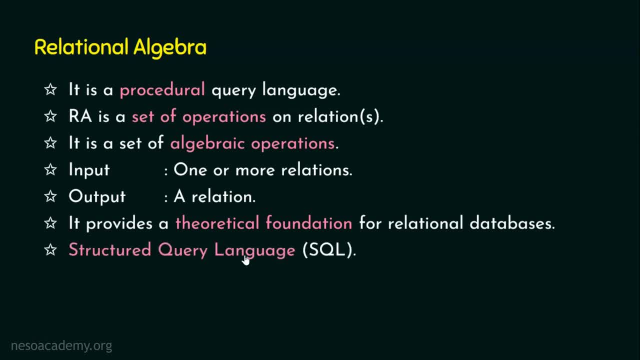 language that is widely used in today's world is the Structured Query Language, SQL, And when you want to become proficient with SQL, knowing relational algebra will give an additional advantage. And not only that, when we have a sound knowledge in the relational algebra. 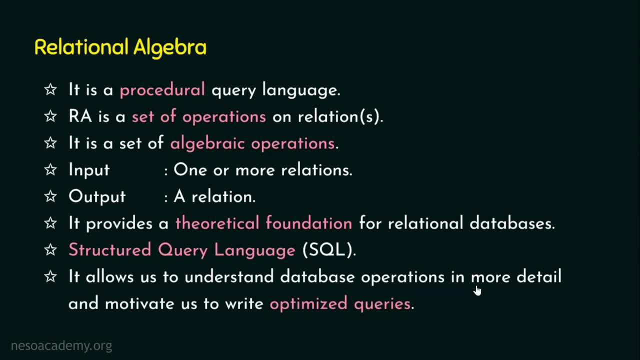 obviously it allows us to know the foundations of the relational database. It allows us to understand database operations in more detail And also it motivates us to write optimized queries. We know databases are going to respond to queries. When we supply a query to 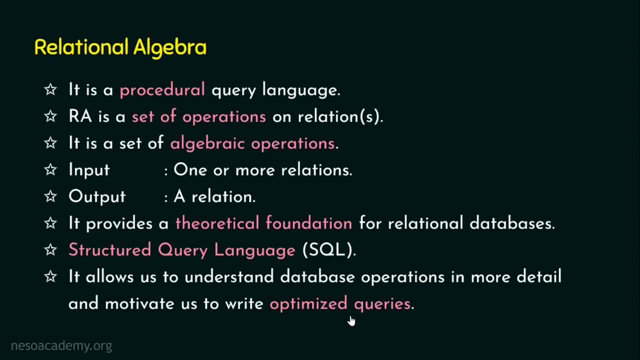 the database. database accepts the query, does the operation and gives the result. If we want to get that output, there may be multiple ways. If we want an output from the database- I mean a relation or a table- there can be multiple queries where these queries gives the same output But giving an 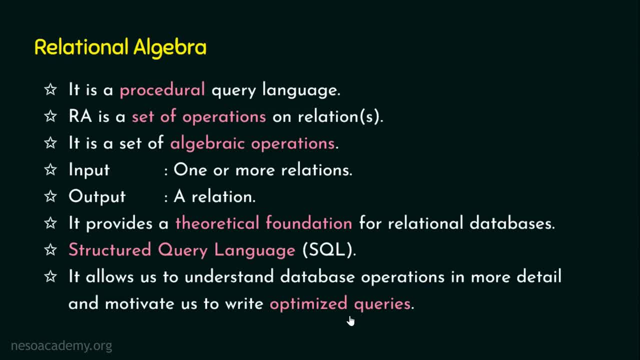 optimized query, we can't get the same output, So we need to know the foundations of the relational algebra. So what I mean to say is, instead of giving a query to the database, if we give an optimized query, the database will respond easily because these optimized queries will be having 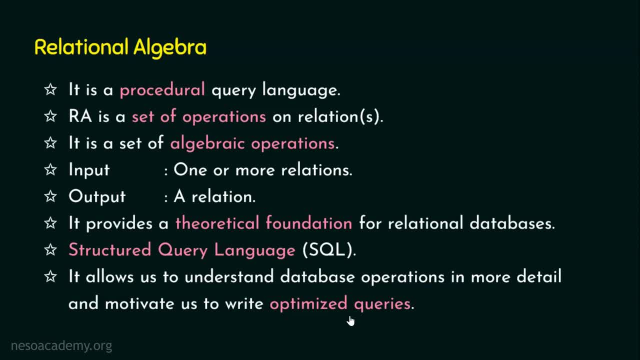 lower cost. Cost is one of the factors that are used to measure the query optimization. In simple terms, relational algebra helps us to write optimized queries And also it helps us to understand the database operations in more detail: What's happening at the backend, how queries are. 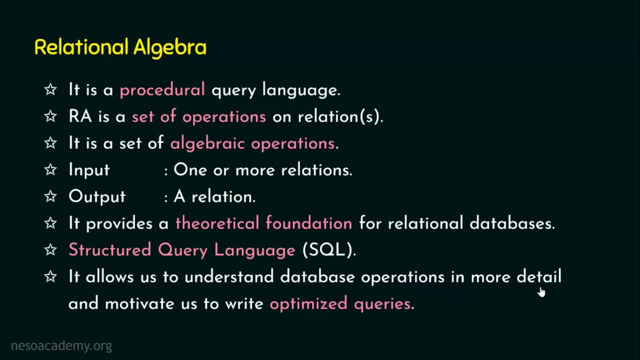 processed, how query execution plans are generated, how the plans are executed, all these things. No worries. in the coming lectures we are going to focus on query optimization techniques. At the time I will explain you how query optimization is actually taken care by database. We are done. 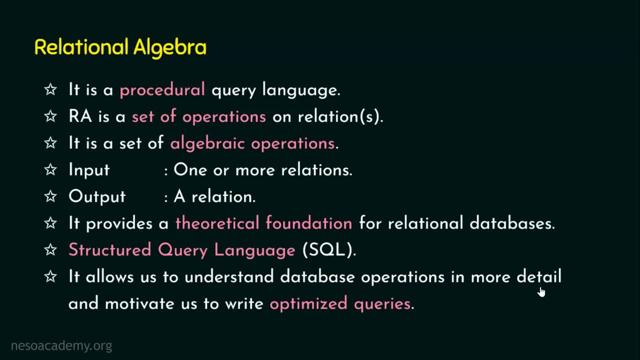 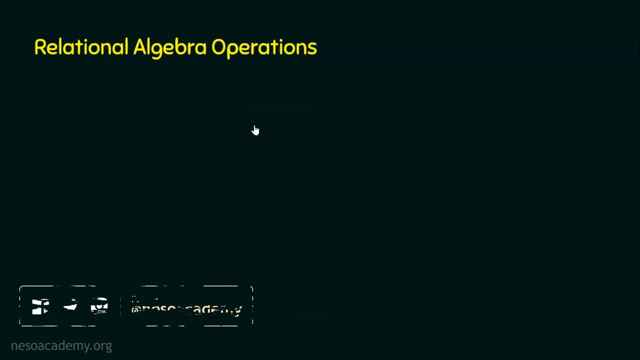 now, Basically, the relational algebra operations are classified into two categories: Number one, the fundamental operations, and number two, the additional operations. Let's just focus on the names of the operations in this lecture. In the coming lectures we are going to focus on all the 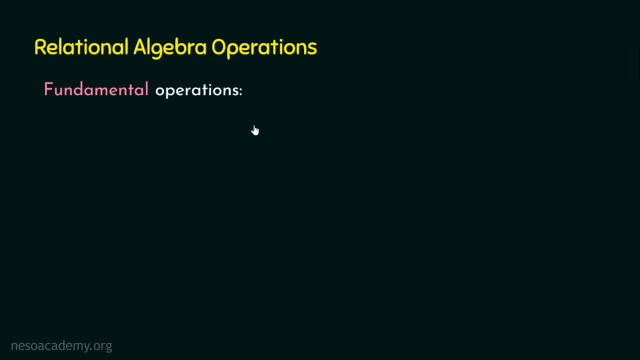 operations one by one in detail, with required examples. For now, let's just know the operation names. Talking about the fundamental operations, we are going to focus on the operations of the fundamental operations. There are six fundamental operations as far as relational algebra is.